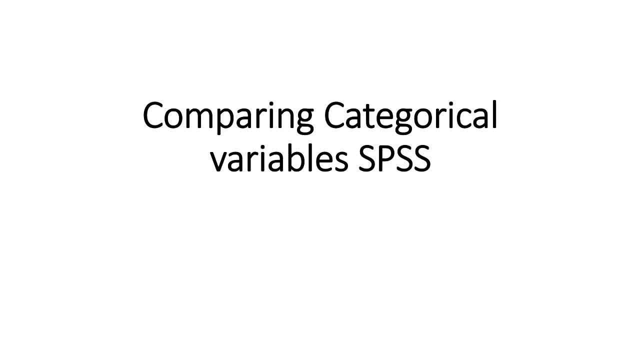 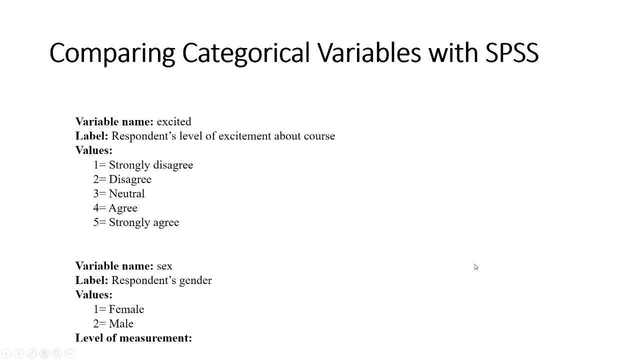 Hi guys, in this video we're going to be comparing categorical variables using SPSS. So often times you'll find yourself in the situation where you want to compare two categorical variables. In this case, we're going to be using two variables from the class survey. We're going to be using the variable excited, which corresponds to the respondent's level of excitement about the course. 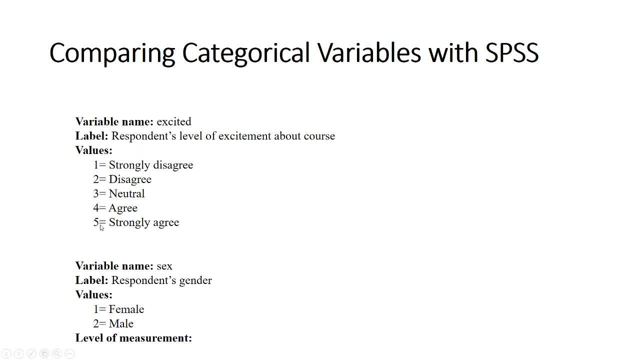 This is a categorical variable that ranges from 1 to 5, strongly disagree to strongly agree, And we want to know specifically whether or not there are differences between males and females in their level of excitement about the course. So whenever you want to compare categorical variables, you must use a cross-tabulation table. 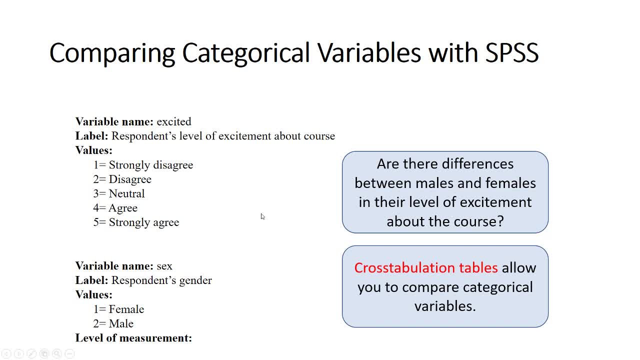 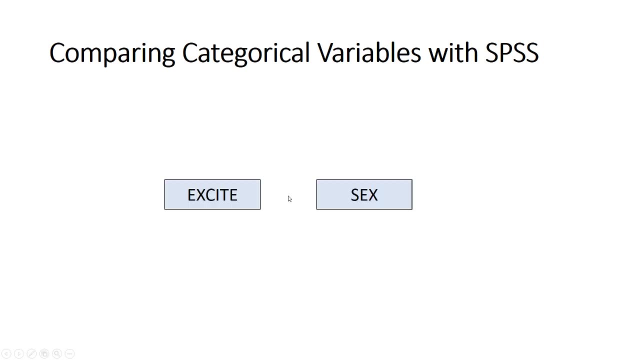 Essentially, what a cross-tabulation table does is that it allows you to see how one categorical variable is distributed across the values of another categorical variable. Again, just like comparing averages between groups, you have to before you can go to SPSS. you have to determine which of the two variables that you're comparing is the independent and dependent variables. 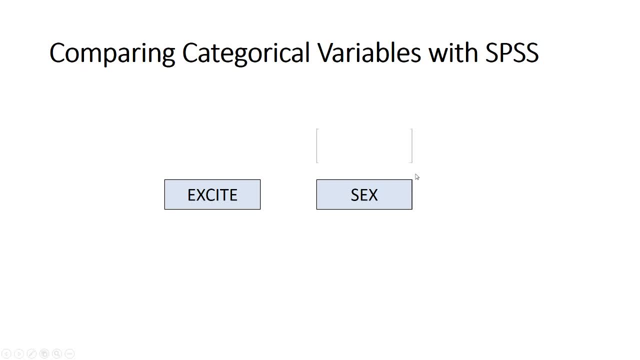 Of course, in this case, just like the last one, sex happens to be the only plausible independent variable, because your gender might influence how excited you are about a math or statistics course. However, how excited you are about your course or a particular course cannot influence your gender, because your gender is already set. 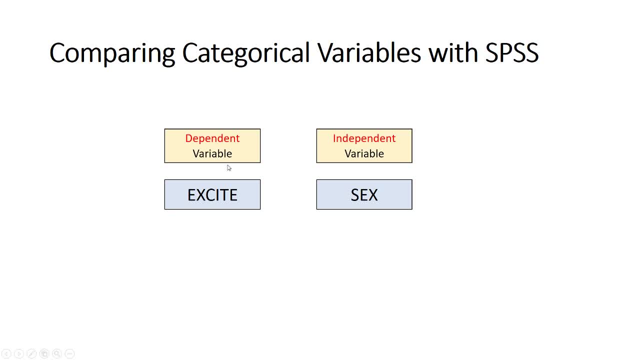 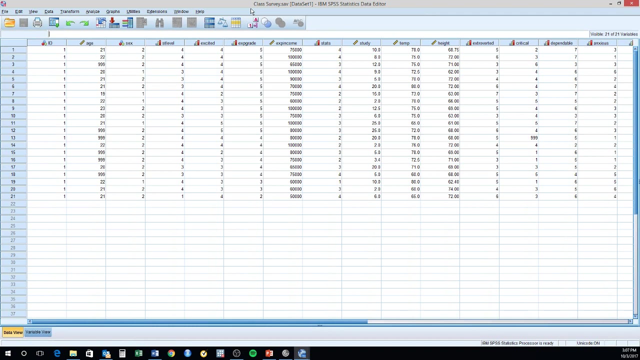 So therefore, excited is the dependent variable. gender is the independent variable, You must know this coming in. So now that we got that out of the way, we can go to SPSS and carry out the analysis, So to compare categorical variables. 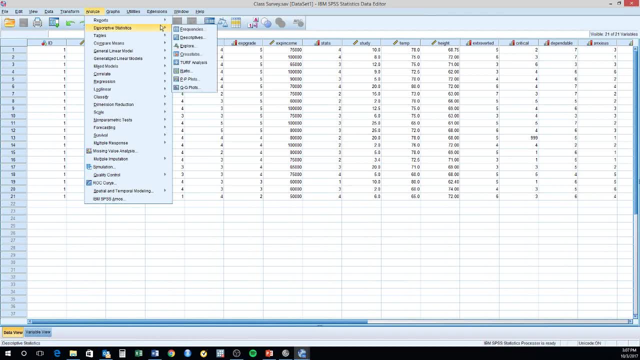 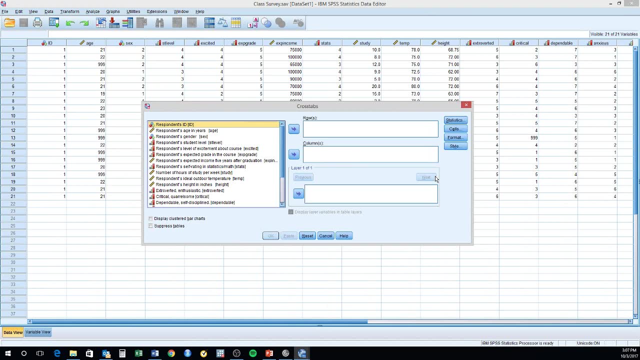 you're going to go to analyze descriptive statistics. you're going to go to cross-tabs. Now, determining which one is the independent variable, which one is the dependent variable is important, because it will allow you to know where to put the variable.